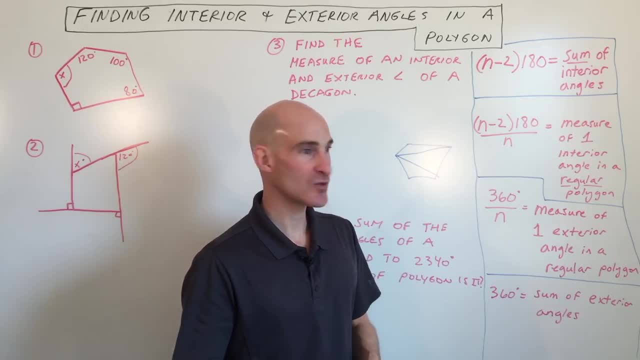 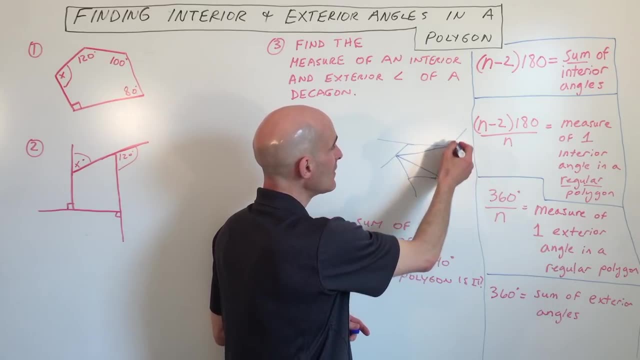 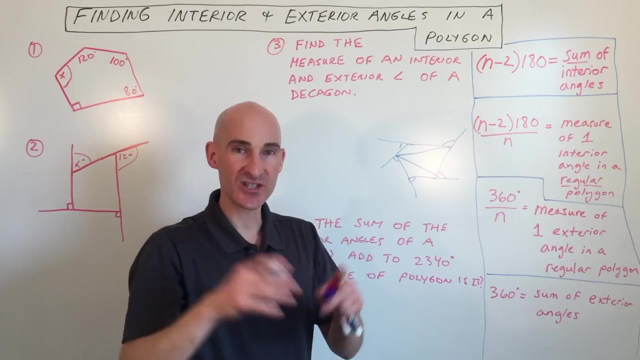 always going to add up to 360. it doesn't have to be regular, they just they're always going to have to 360. so, for example, here, if I extend, you know the sides like, so these angles that are formed on the outside of the polygon here, okay, those are all going to add up to 360 like a circle, okay. so 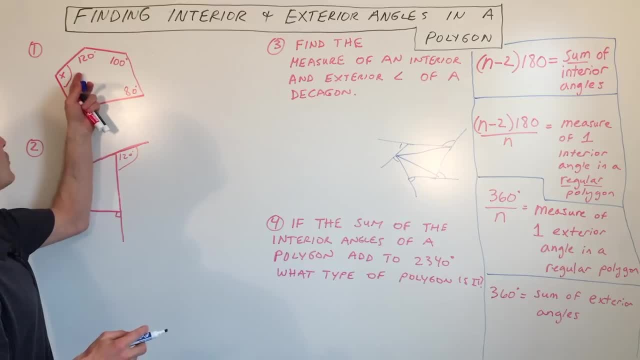 let's get into some examples. I'll show you how these work, excuse me so. and this polygon. here you can see we have one, two, three, four, five angles. or you could count the sides: one, two, three, four, five sides. so we're gonna do m minus two times 180 equals the sum of the angles. so we have five. 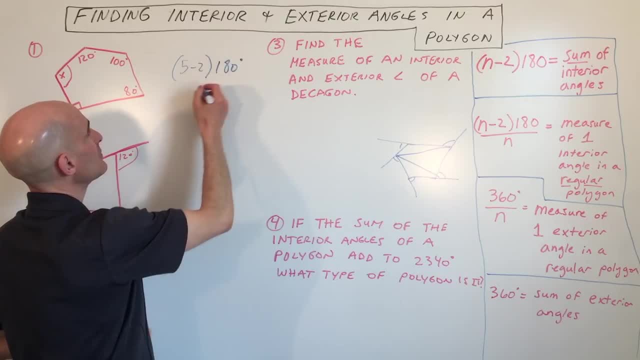 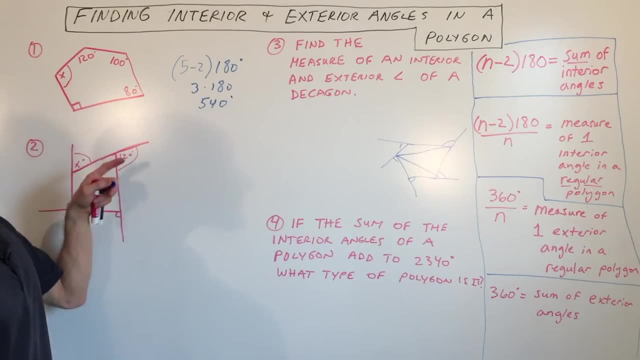 minus two times 180, which is three times 180, which is 540. okay, so if we want to solve for X, this missing angle here, we're going to add up all these angles, angles, okay, plus x equals the total 540.. So let's do that. So that's 120 plus 80 is 200,. 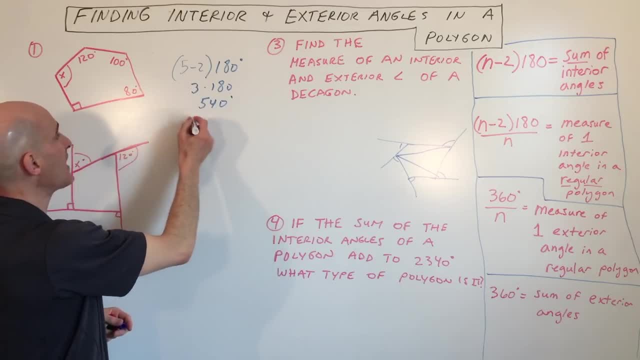 plus 100 is 300, plus this right angle here, that's 90, that's 390.. So we have 390 plus x equals 540.. So if we subtract 390, what do we get? We get 150 degrees. So that's this angle right. 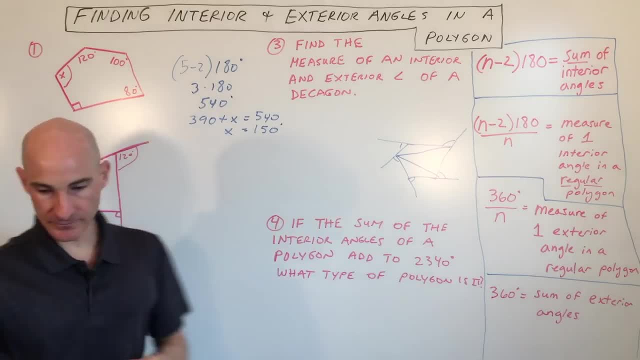 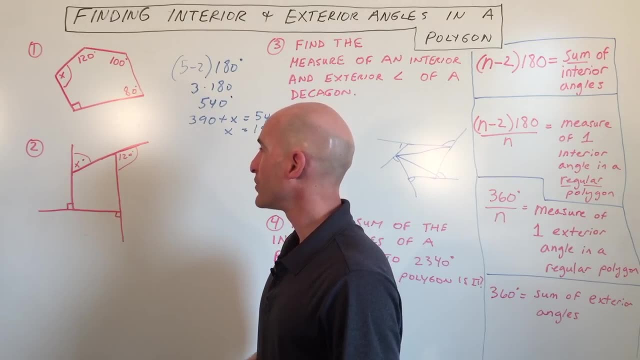 here. Now, in this one here- excuse me, in this angle, in this polygon, here, we're trying to solve for the exterior angle. So what we're going to do here is we're going to add up all the angles, okay, and the exterior angles add up to 360.. So in this one we're just going to go over. 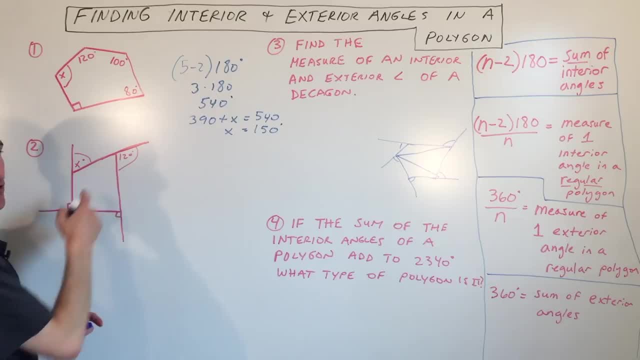 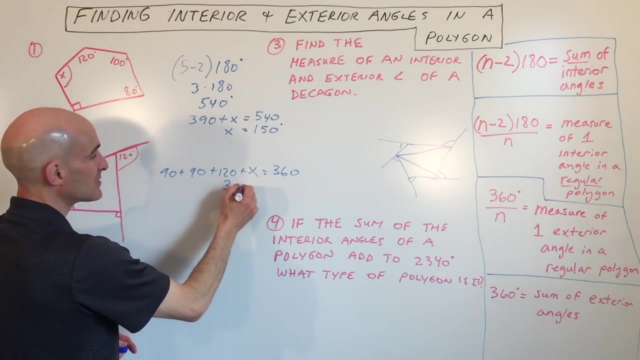 here we're going to say: all right, 90 plus 90 plus 120,, that's 90 plus 90 plus 120, plus x, this angle here equals 360.. So that's 180 plus 120 is 300, okay, so 300 plus x equals 360,. 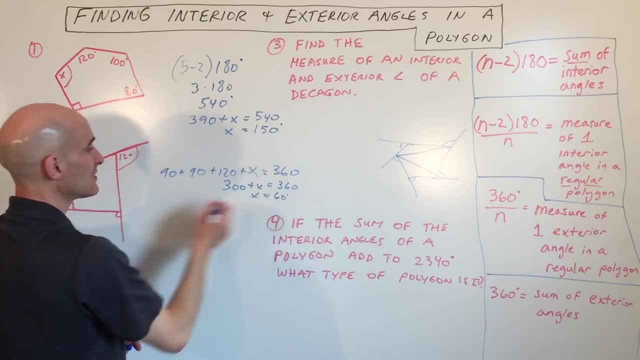 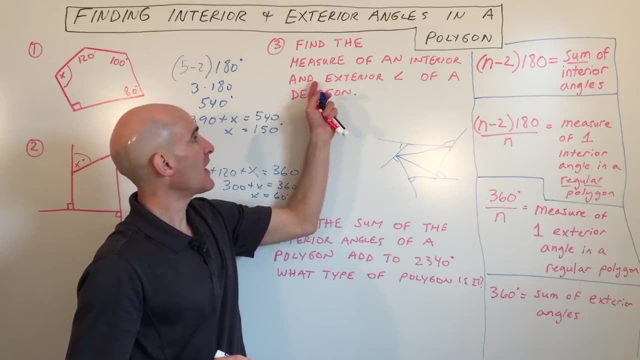 and if we subtract 300, we can see that x equals 60 degrees. that's this angle, right here. Okay, now the next one. find the measure of an interior and an exterior angle of a decagon, and what I meant to write here is a regular decagon, So I'll just put that in there. 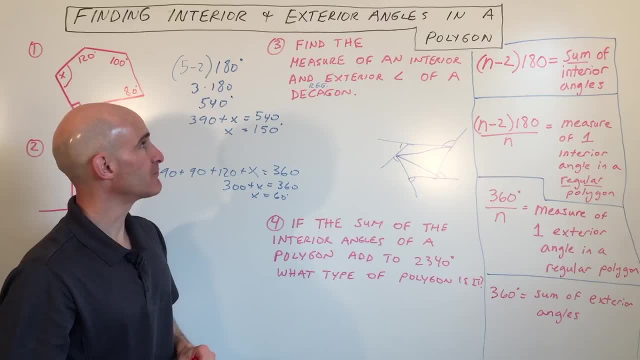 regular decagon, meaning all the angles. All the angles and all the sides are the same. So a decagon is like decade. right, there's 10 years in a decade. there's going to be 10 angles in a decagon. So there's a couple different ways to do. 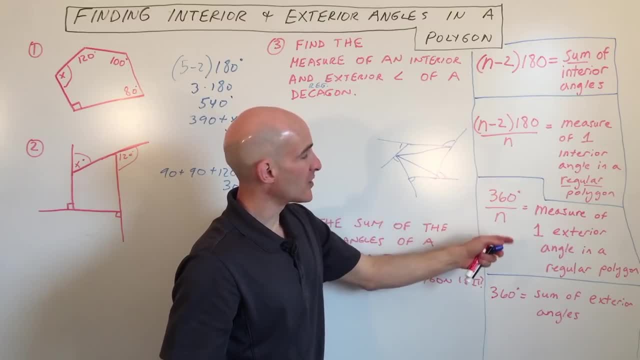 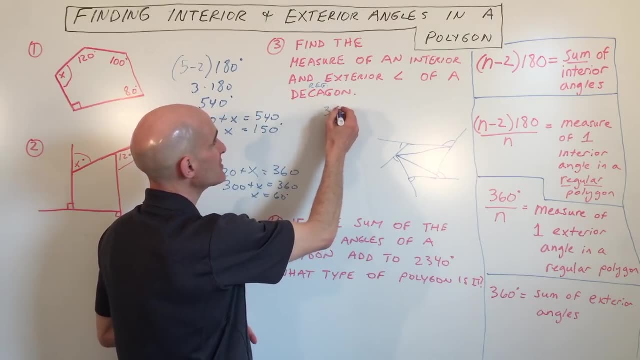 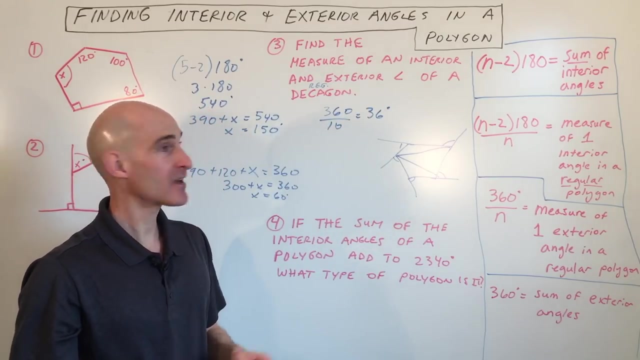 this. We can either use this formula here or we could use this formula here. I'm going to use this one here. it's going to be a little bit easier, since it's a regular decagon. So I'm just going to take 360 divided by 10, that equals 36 degrees, So each of the exterior angles of that decagon. 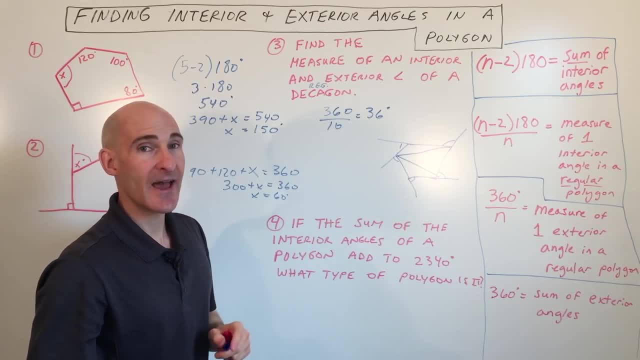 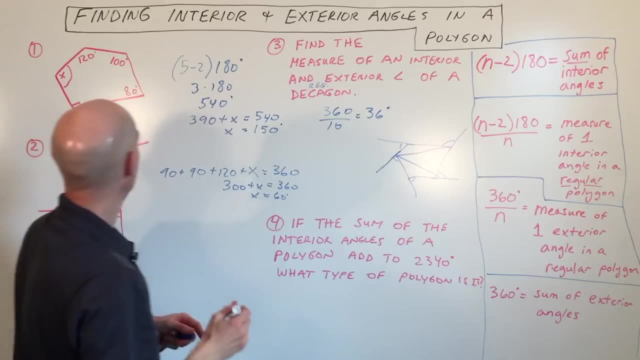 will be 36 degrees. But one thing that you'll notice is that, see, when you extend this side, okay, like this, the interior angle and the exterior angle, they're going to be supplementary. This might be a little bit easier to. 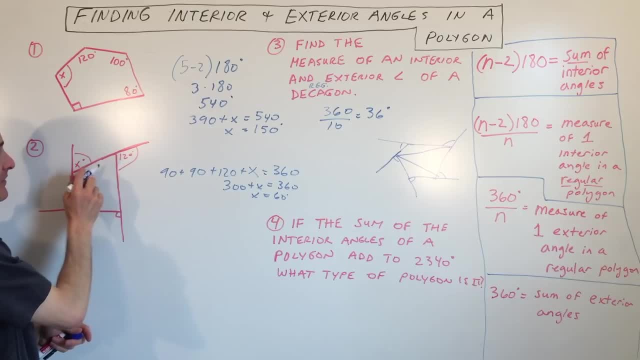 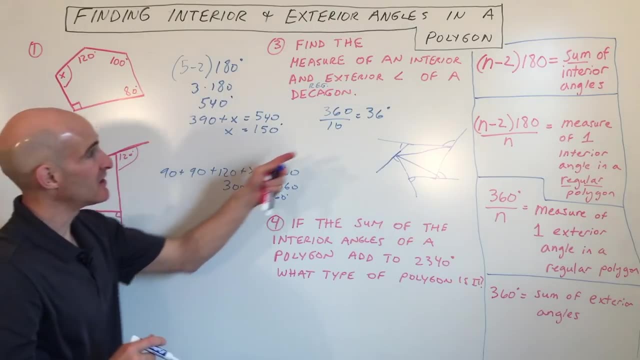 see here. So when I extended that side, the exterior angle and the interior angle, see how they form a line, a linear pair. they're going to add up to 180.. So if this is 120,, this is 60.. If this is 36,. 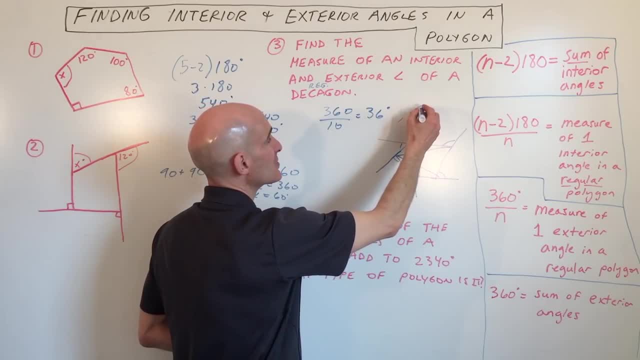 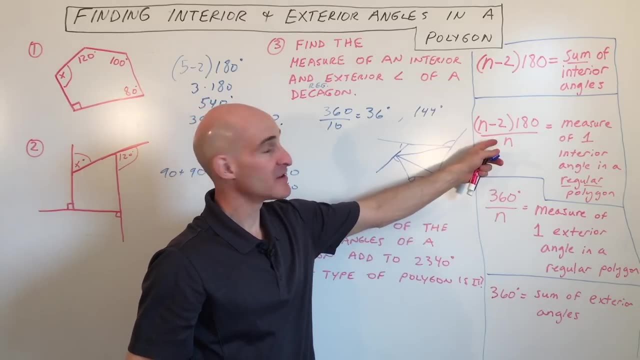 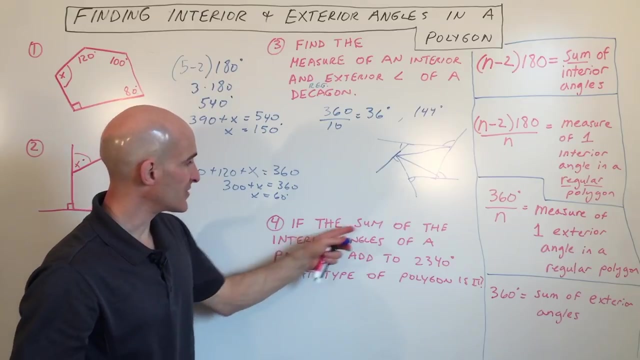 right. the interior angle would be 180 minus 36.. So that's 144.. Okay, so sometimes it's easier to use this formula than this formula. It's just a little bit simpler if it's a regular polygon, right? Okay? so then the last one. if the sum of the interior angles 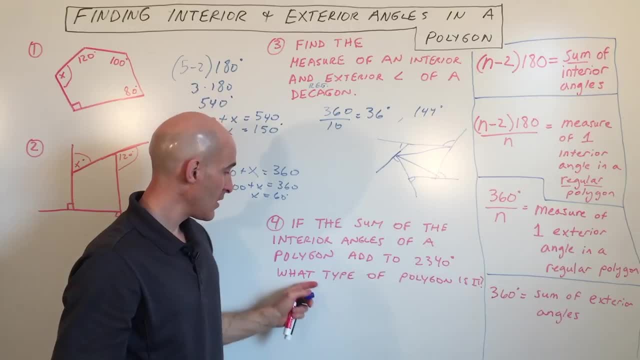 of a polygon add to 2340,. what type of polygon is it? Okay, so this one. it doesn't specify whether it's regular or not. It just says that all the interior angles add up to 2340.. So we're going to. 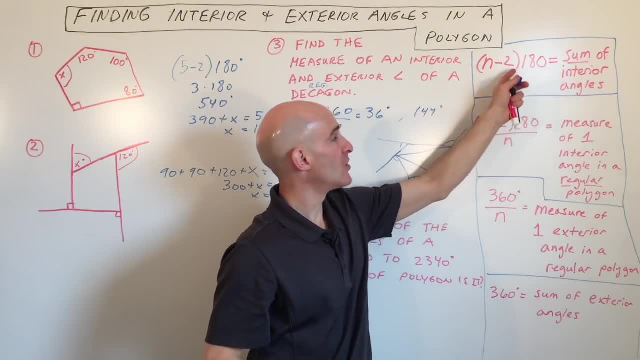 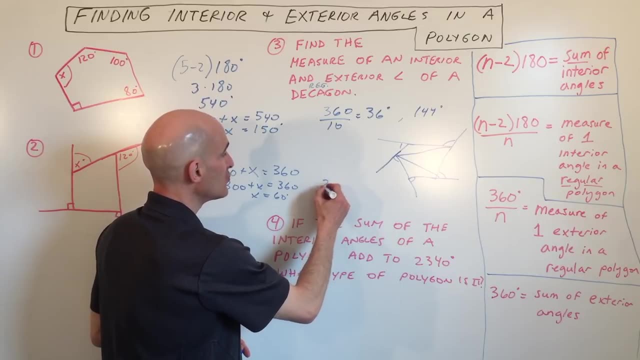 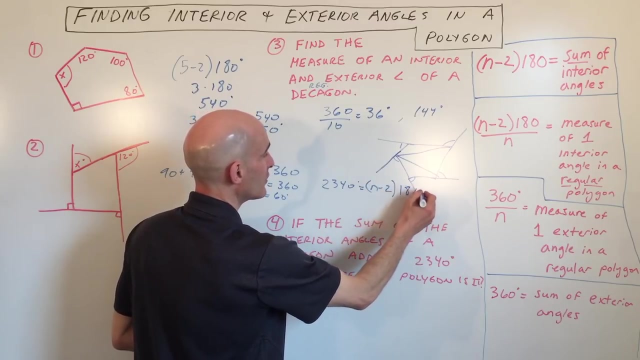 go to this formula here: the sum of the interior angles. So it's helpful to you know. memorize these formulas, if you haven't already, And let's see if we can substitute what we have. So we have 2,340 equals n minus 2 times 180.. Okay, I'm going to divide both sides by 180.. 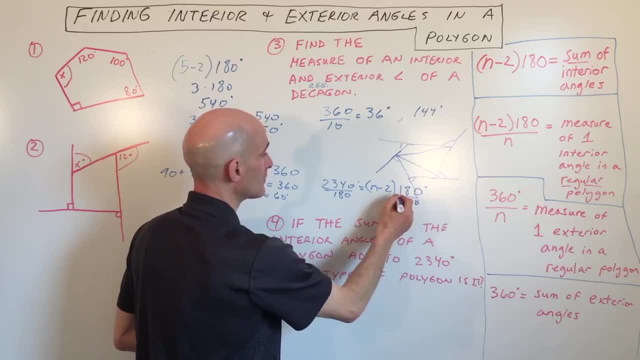 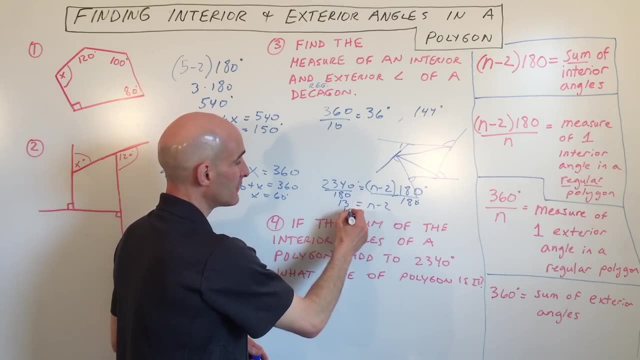 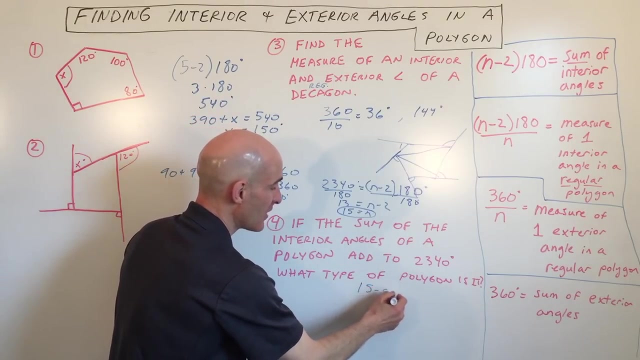 Okay, This comes out to 13.. And then if I add 2 to both sides, I get 15 equals n. So this is a 15 gone, Okay. So when it starts to get up in those higher numbers, you can just put 15 dash gone. 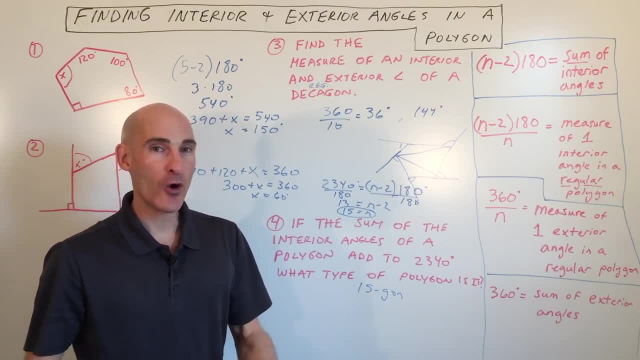 15 sides or 15 angles dash gone. So I hope you've been enjoying these videos. I hope you learned something. Sometimes it's just a little, you know piece that's missing that can make a big difference in boosting your growth. So I hope you've been enjoying these videos. I hope you